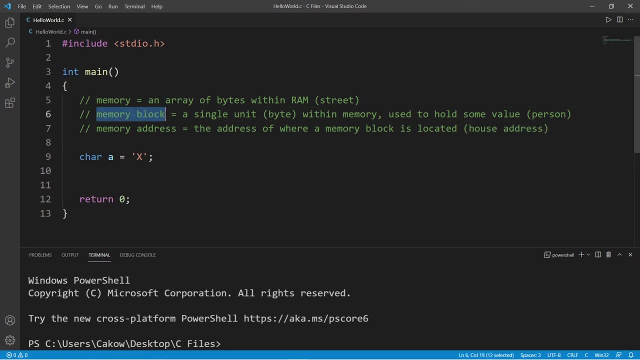 address. If I were to open their front door, I should probably knock first. at least then I will find the character I'm looking for. If I were to go into their front door, I should probably knock first. at least then I will find the character I'm looking for. If I were to open their front door, I 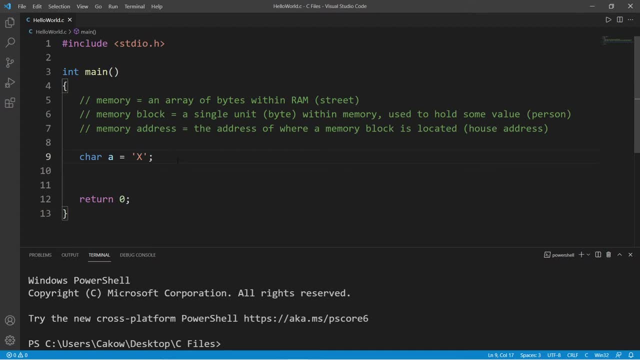 character x. So that's kind of an analogy I like to use when thinking about memory. So let's declare a couple other characters. We have char b- I'll give this a value of y- And char c And I'll give this a character of z. Okay, so let's find the size of each of these characters. So I'm going. 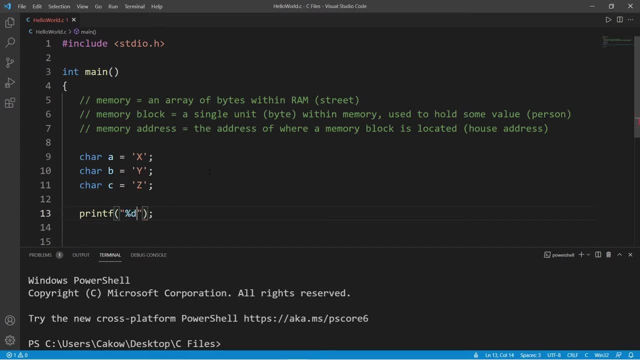 to use a printf statement. I'm going to display an integer And the size of each of these characters is within bytes. So I'm going to use the size of operator and pass in one of my characters. So I'm going to pass in a, And I'll do the same thing with b and c. So the size of each of these. 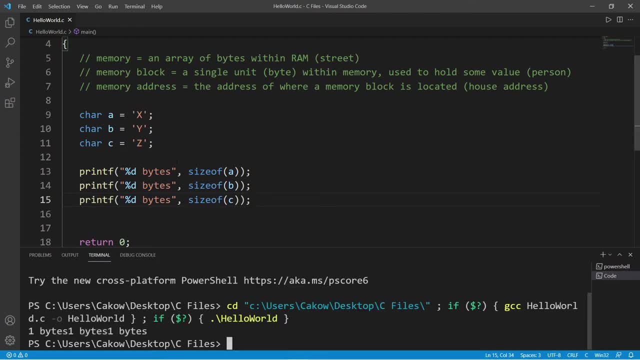 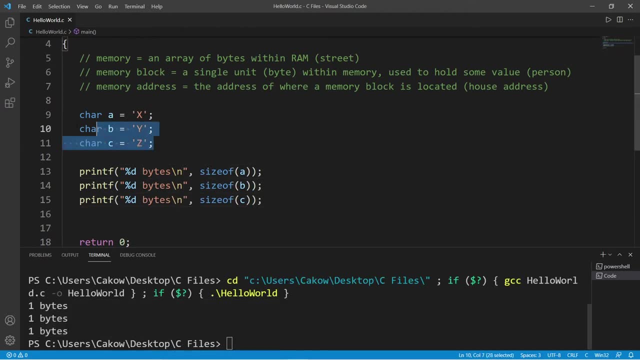 characters is one byte, And I think I'm just going to add a new line here. Much better, Okay. now we can actually access the address of each of these variables. So each of these variables is using one block of memory. A single block of memory is a byte. 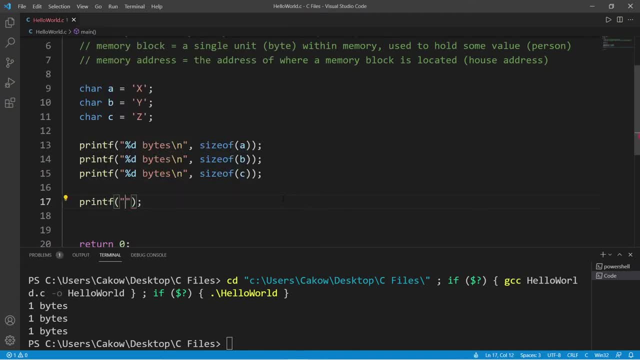 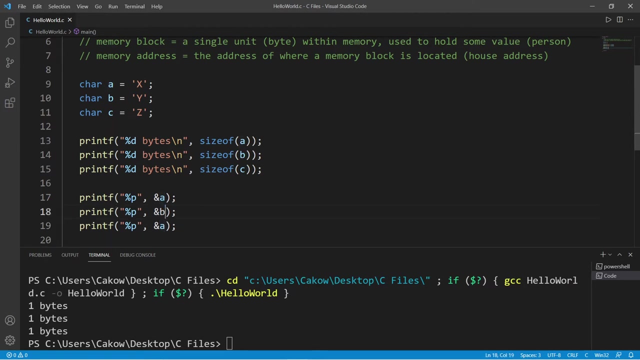 So within a printf statement I would like to display an address, So the format specifier is p And I will use the address of operator, then the name of one of my variables. So I'll display the address of variables a, b and c And then display each on a new line. 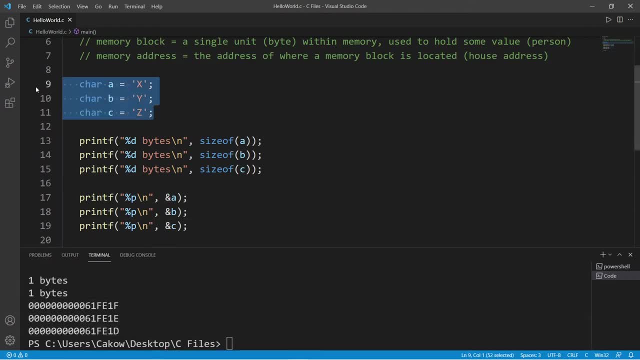 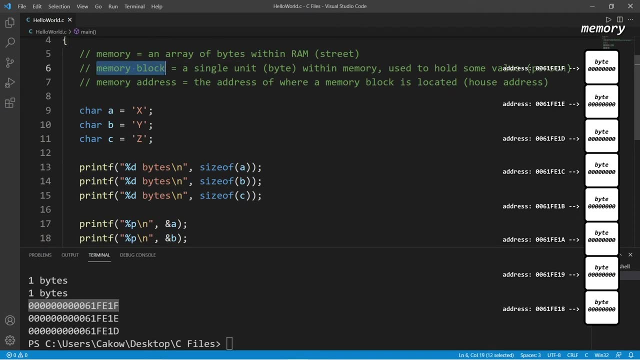 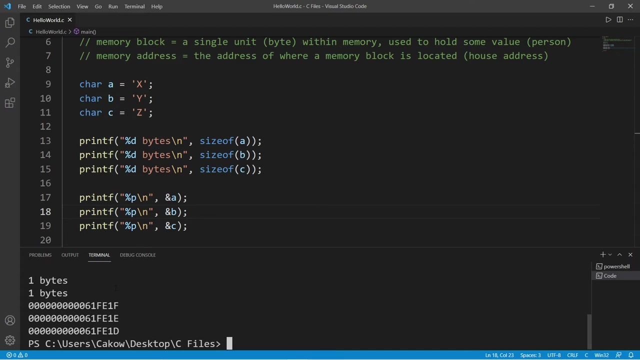 So here are the memory addresses for these three variables. These addresses are in hexidecimal. These are the street addresses of each of our memory blocks on our fictional street. Hey, so this is bro from the future. Just a quick crash course on hexidecimal values With standard decimal values. 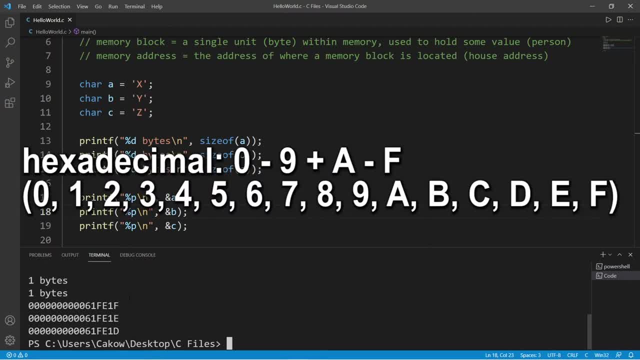 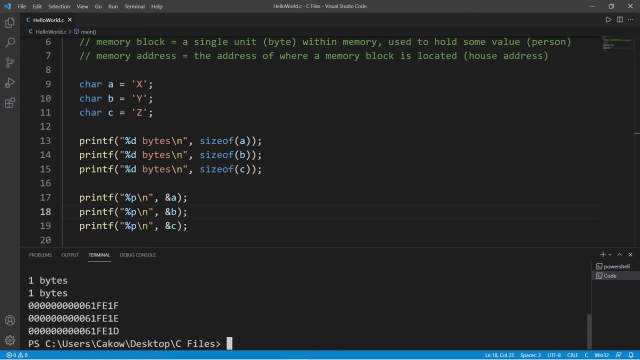 they use the numbers 0 through 9.. But with hexidecimal you use the numbers 0 through 9, as well as a through f, So that gives you a total of 16 different values for each digit. So that's why there's a mix of numbers and letters. 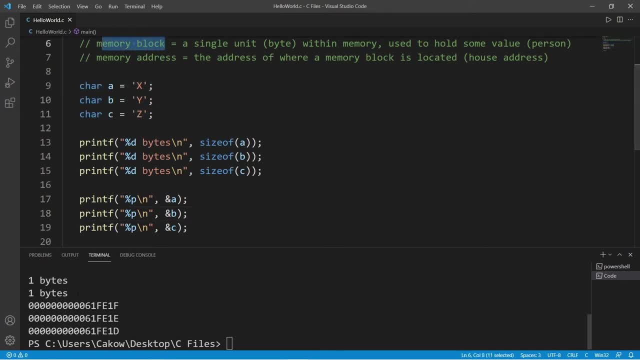 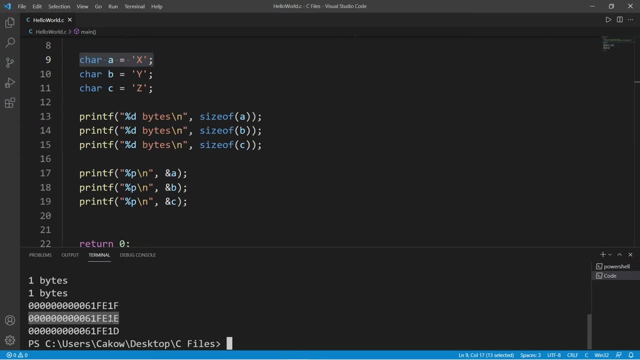 So each of these variables uses one memory block. They use one byte of memory. So, beginning with variable A, this has this street address. But if we go down to the next memory block you can see that there is just one change: F goes down to E. and then with variable C. 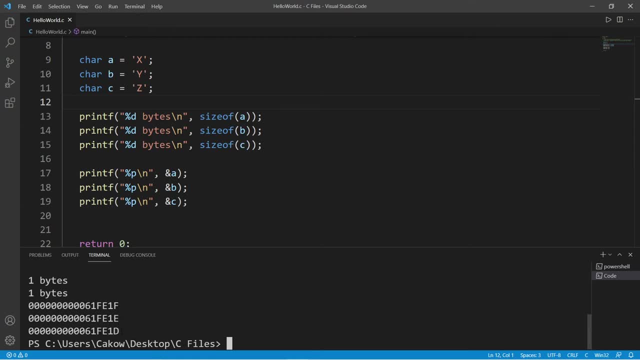 this address goes down by one. So F E, D, these are contiguous memory blocks. They're all next to each other. But now if we switch to a different data type, like a short? we haven't used these in a long time. 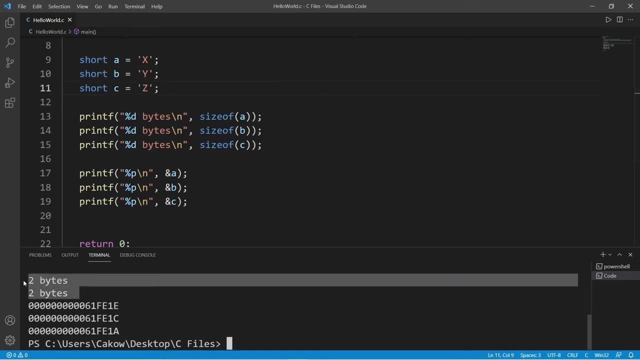 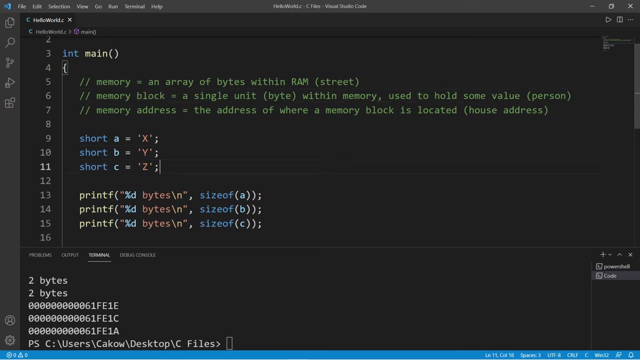 Well, shorts use two bytes of memory, as we can see here. So these hexadecimal addresses are now going down by two: E, D, C, B, A. So each of these variables are using two memory blocks. We need an even larger house. 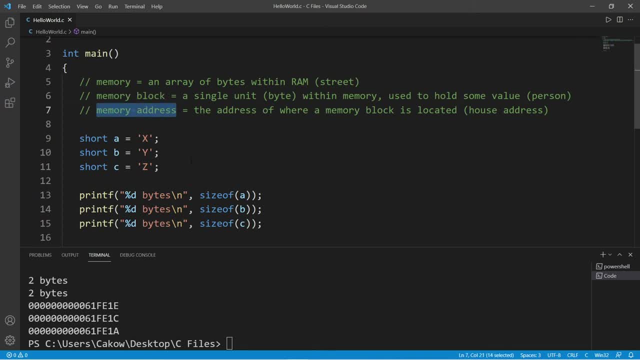 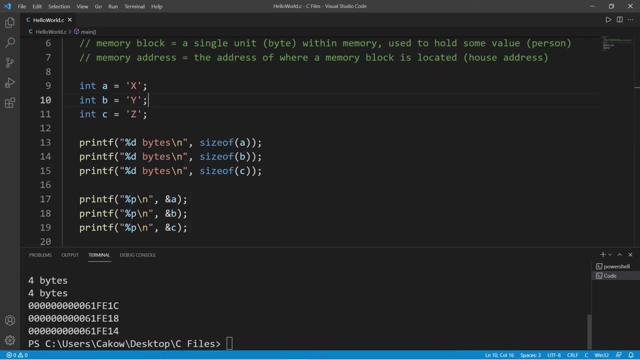 Even more memory blocks And they use up two memory addresses. And then if I change these to integers, well they're going to use up even more memory. So integers use four bytes of memory. And these are the street addresses of these three variables. 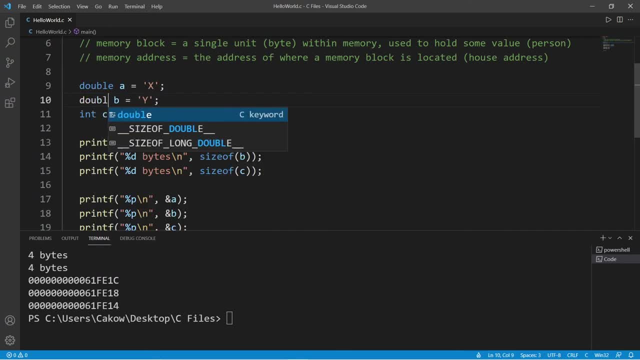 And doubles, use double the size of an integer. Doubles, use eight bytes of memory, And these street addresses are decrementing by eight. If this was a fictional value, then that would be equal to eight. If this was a fictional value, then that would be equal to eight. 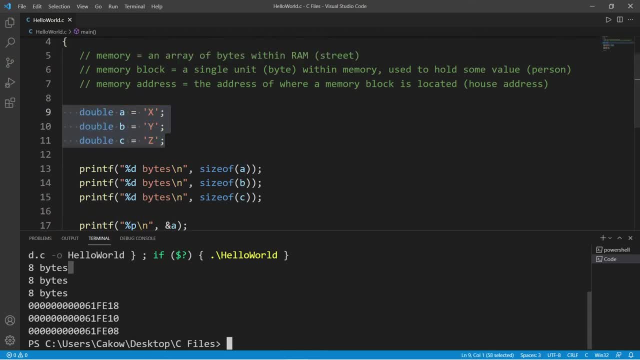 street with houses. well, doubles use up 8 bytes of memory. So think of these like mansions. They're using up a lot of space. Now, what happens with an array? I'm going to declare char a and declare an array. This will be an array of characters to begin with. So let's say: 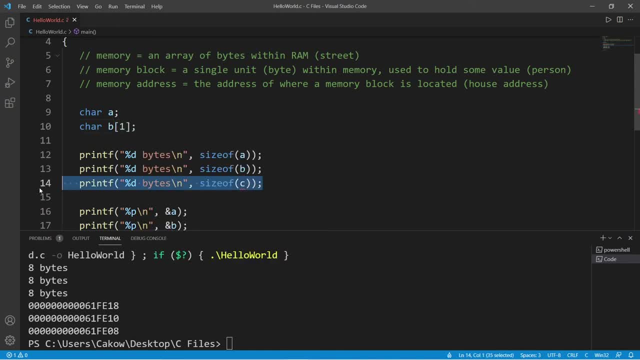 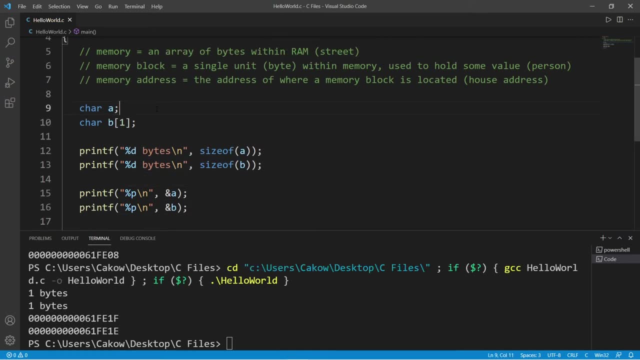 character array b, and I'll give this a size of 1.. So I'm going to print the size of a and the size of b as well as their memory addresses. Our single character a uses 1 byte and this is the street address of this variable and our array b. 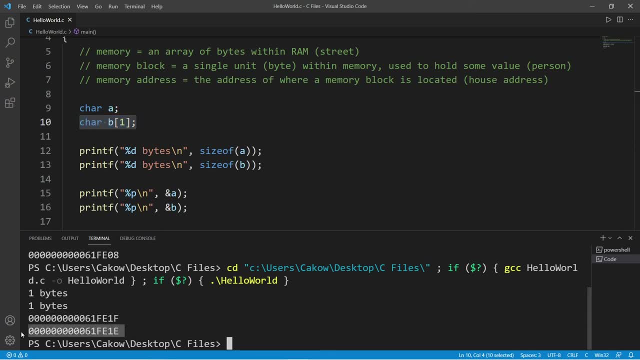 also uses up 1 byte, and this is the street address of where this array begins. If I set the size of this array to 2,, well then my array is going to use 2 bytes and now it has a different address to accommodate the increased size of the array.